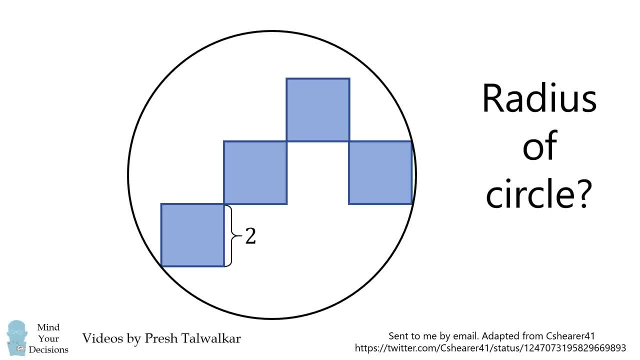 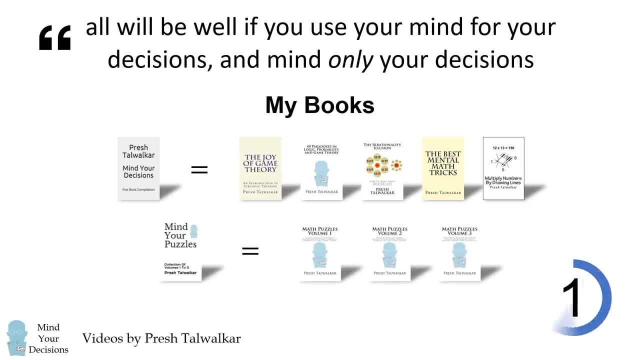 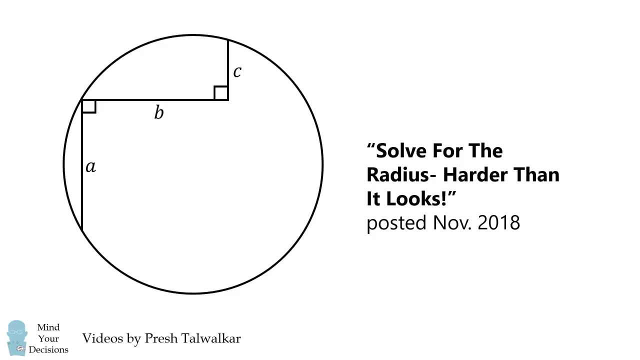 Pause if you'd like to give this problem a try and, when you're ready, keep watching to learn how to solve this problem In the video. Solve for the Radius. Harder Than It Looks. the challenge was to solve for the radius of the circle in terms of the lengths A, B and C. 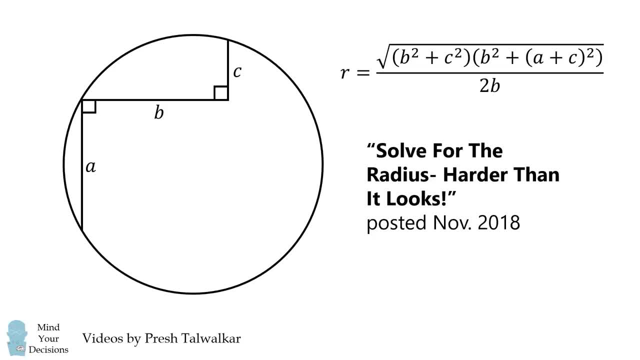 We derived the following formula. In this video, I'm going to prove this formula once again, and then we will use this formula to solve the original problem. Let's get started. Draw a horizontal length equal to B. Then draw a vertical length that connects to the circle By symmetry. this length must be equal to C. 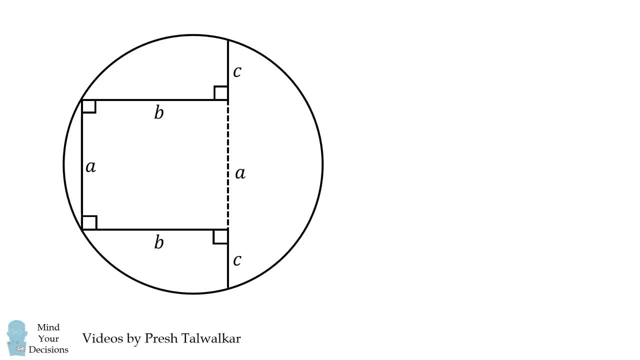 We then connect these two line segments and this length will be equal to A. We then extend the line segment with a length of B to the other side of the circle and label this length as D By power of a point or the intersecting coordinates theorem. 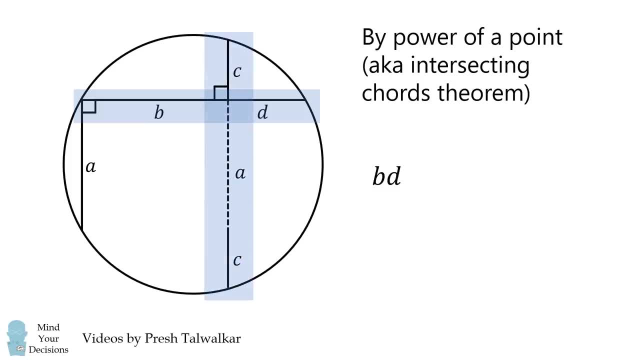 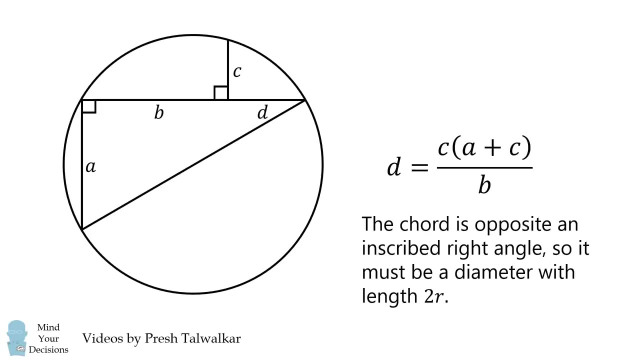 we must have. B multiplied by D is equal to the product of C and A plus C. We divide both sides by B to get the following formula: for D We then draw the following chord of the circle: Notice this chord is opposite an inscribed right angle. 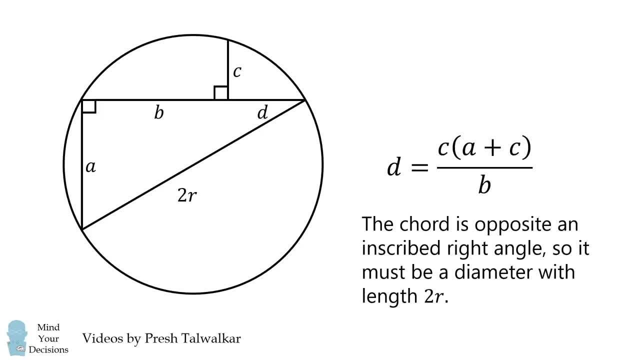 so it must be a diameter of the circle with a length equal to 2R. Then in this right triangle we can use the Gogu theorem. We have A squared plus the quantity B plus D squared must be equal to 2R, the quantity squared. 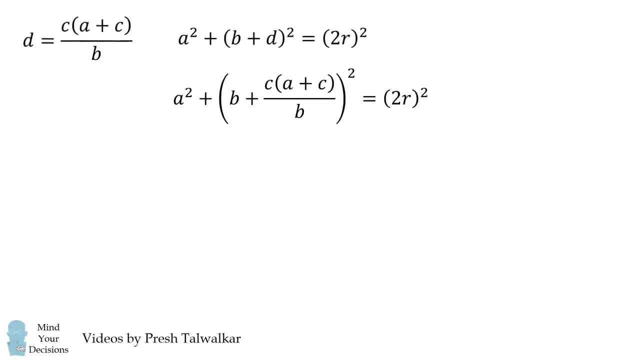 Now let's do some algebra. We'll substitute in for D, then we'll expand out and continue to expand out. We are now going to carefully factor the numerator. We'll do this as follows. The first four terms can be factored as follows: 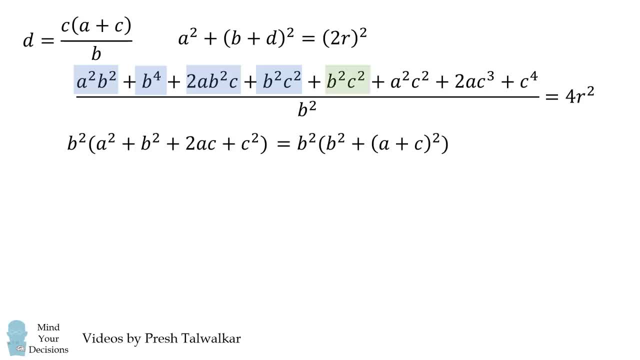 We factor out a B squared and we get the following formula: The next four terms: we can factor out a common factor of C squared. We get the following formula: We substitute those in Now we're going to divide both sides by 4..